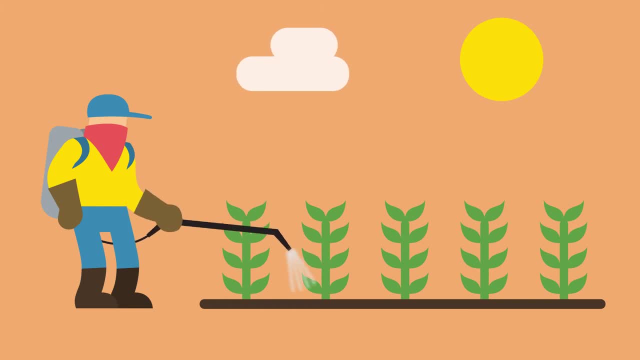 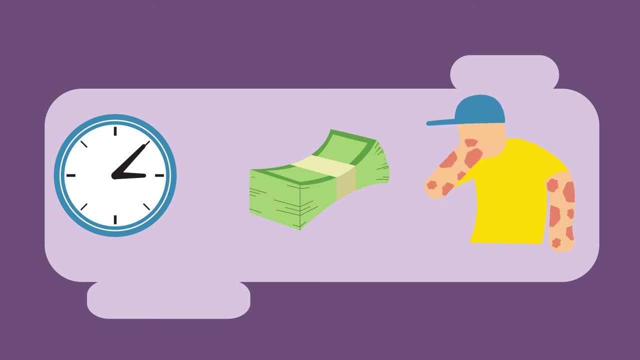 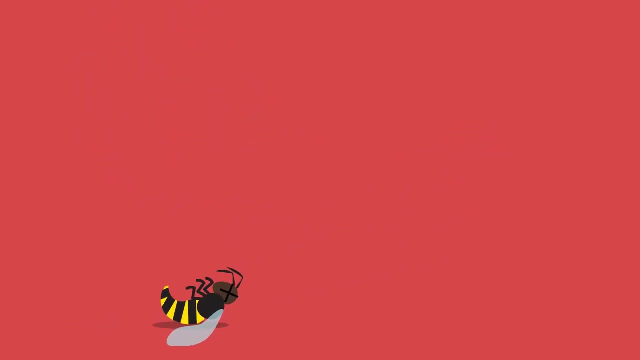 Traditionally, farmers have sprayed their crops with pesticides to kill the insect pests. but this is time consuming, expensive and often harmful to the farm workers in contact with the poisons. Also, pesticides kill useful insects such as pollinators. It can harm other. 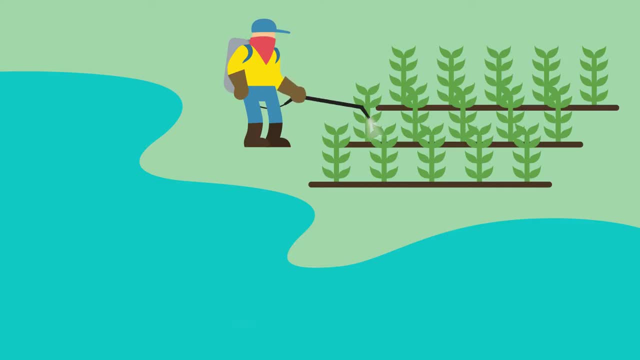 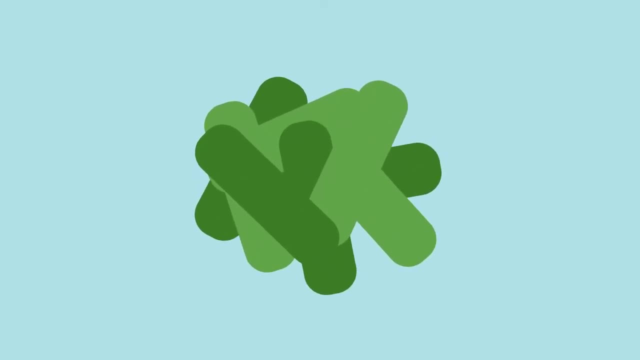 animals that eat the insects that have been poisoned. Spraying the pesticides also damages soil and water in the environment. Crops that are most commonly modified are cotton, soybean, maize and canola. Crops have been genetically modified with a gene from a bacterium called. 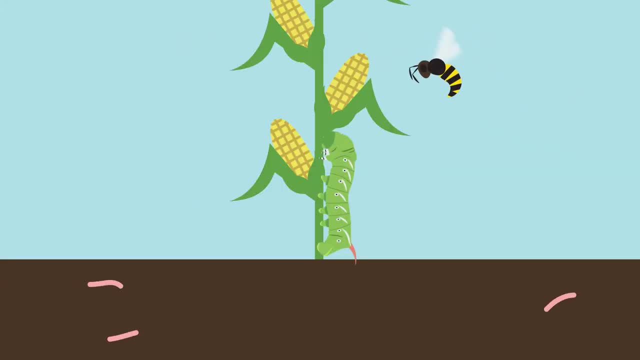 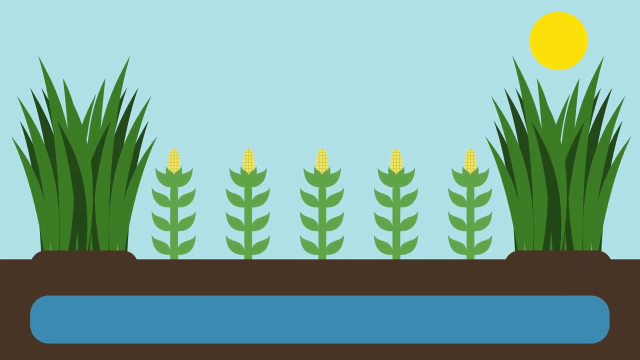 Bacillus thuringiensis. This gene causes the cells of the crop plant to produce an insecticide in their leaves that kills insects that eat it. The genetic modification reduces the need for chemical pesticides. The growth of weeds in fields reduces the yield of crops because the weeds compete with 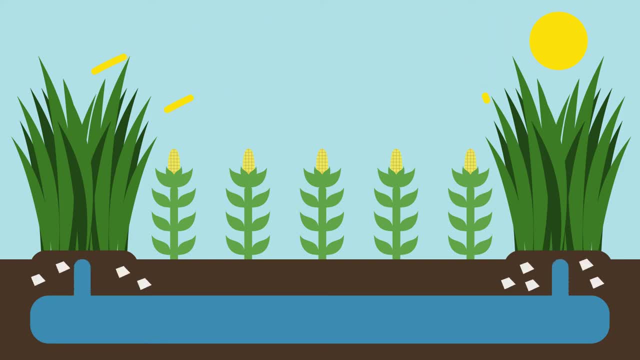 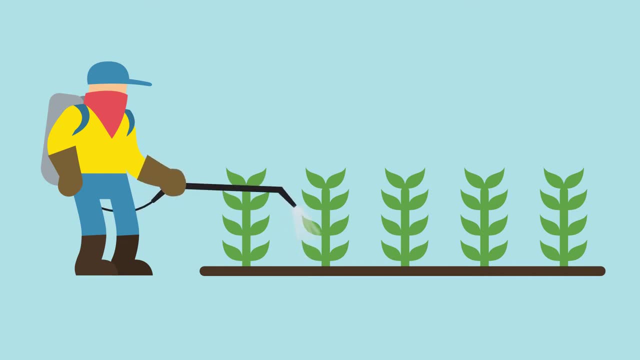 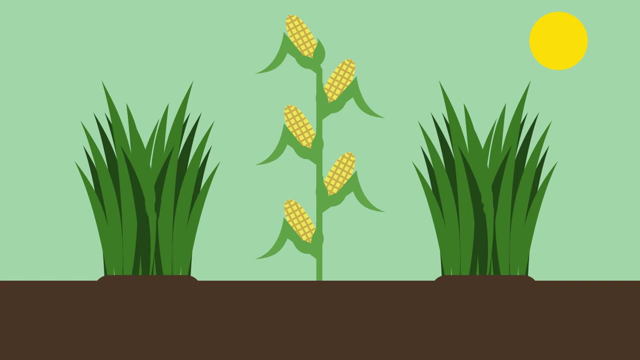 the crops for water, light and minerals in the soil. Plants can spray their fields with weed killers, but this may also damage the environment or even the crop plants themselves. So crops can also be genetically modified to be resistant to weed killers. This means that only the weeds will be killed by the weed killers. 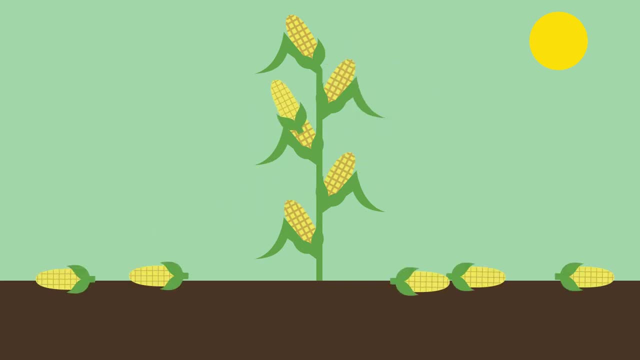 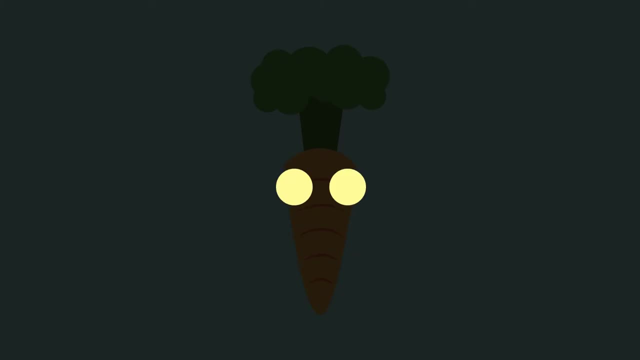 This doesn't reduce the amount of chemicals sprayed on a field, but it does mean that higher yields can be gained. Have you ever been told that eating carrots helps you see in the dark? This is because carrots are a good source of vitamin A, which is essential. 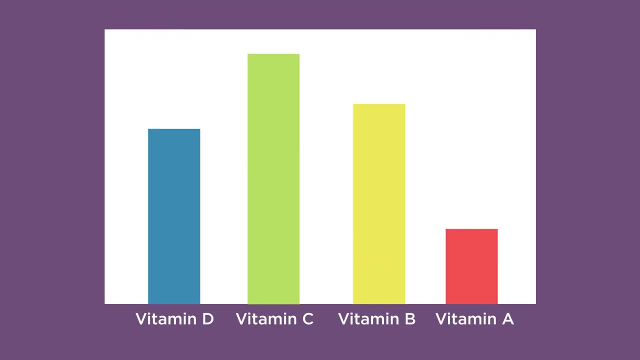 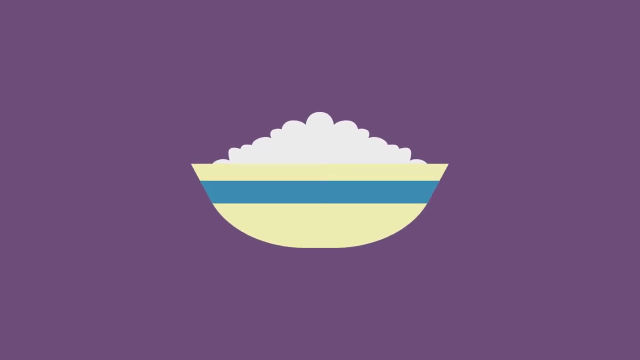 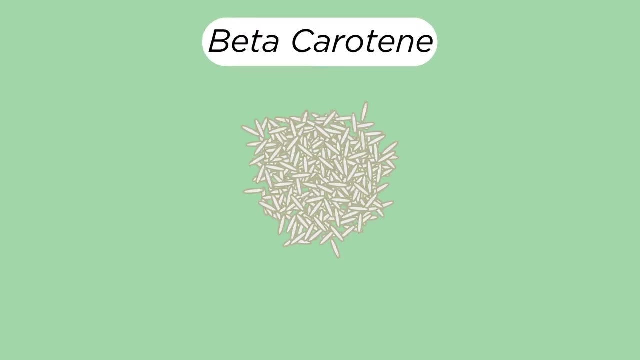 for healthy vision. A common problem in some countries is a deficiency in vitamin A, because people have a diet mainly made up of cereals like rice, with few fresh fruits and vegetables. To overcome this vitamin A deficiency, rice has been genetically modified to contain beta-carotene, which is used in 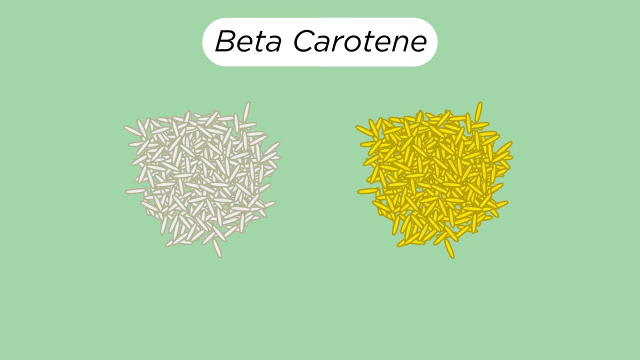 the body to make vitamin A. This gives the rice a yellow color, so it's known as golden rice. Its taste is not altered, but it contains extra nutritional benefits. Other examples of GM crops include those that grow in difficult conditions such as droughts. 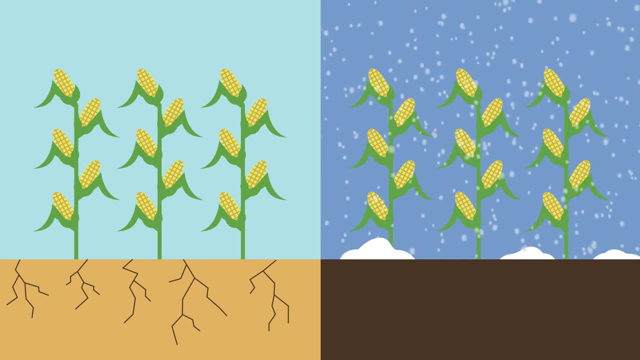 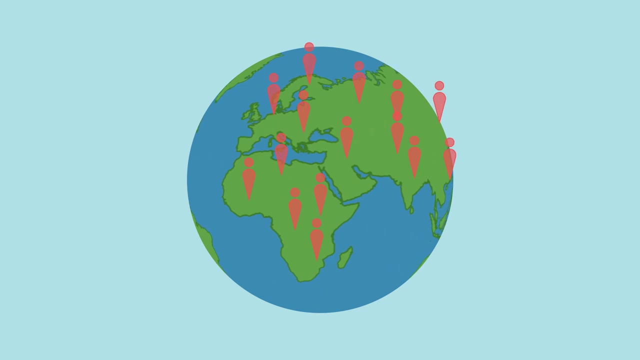 or cold temperatures, and crops that are resistant to diseases. All of these genetic modifications mean we can either increase yields from existing farmland or we can farm low quality land, both of which help us to feed the ever-growing world population, But so far we have only